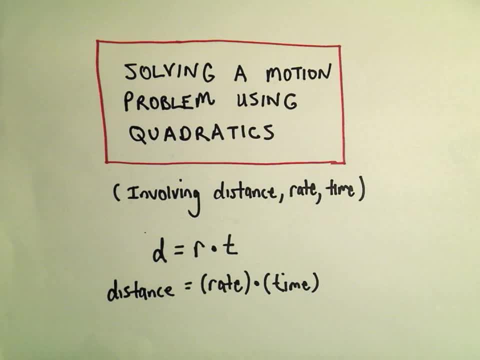 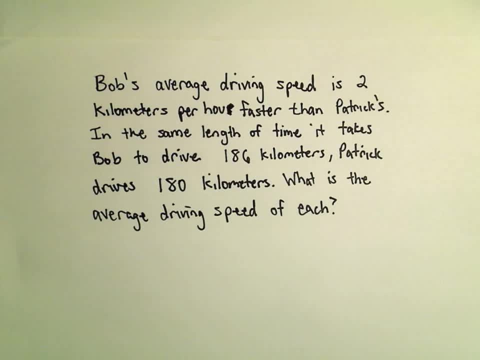 total distance would be 120 miles. Okay, so we're gonna make use of this. So in our problem here we've got that Bob's average driving speed is 2 kilometers per hour faster than Patrick's And the same length of time it takes Bob to drive. 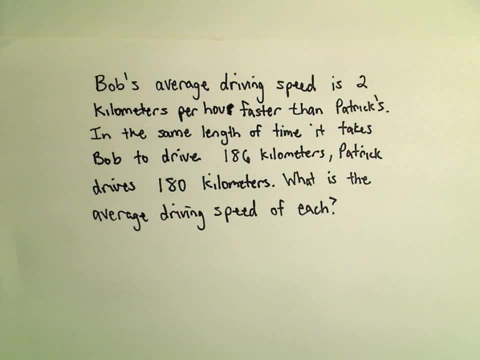 186 kilometers. Patrick's able to drive 180 kilometers, And we want to know what's the average driving speed of each. So what I'm going to do is make two little equations here. So we've got Bob and we got the one relating the information for. 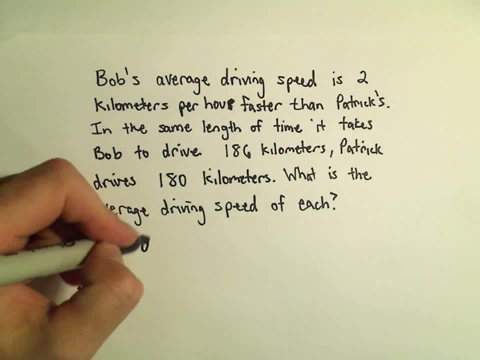 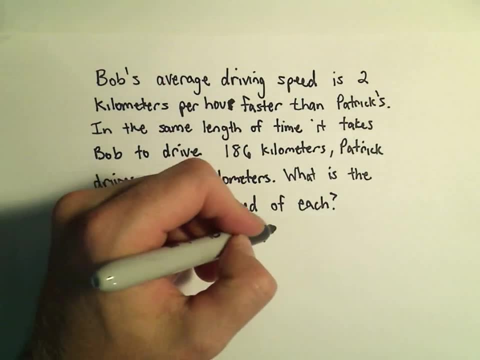 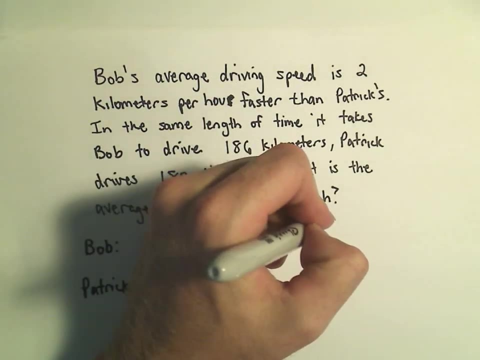 Patrick. Okay, so again we're going to use distance equals rate times time. For Bob here it says the distance he travels is 186.. The rate or his speed? that's what we don't know. So I'm going to write a little r and I think I'm going to put a little. 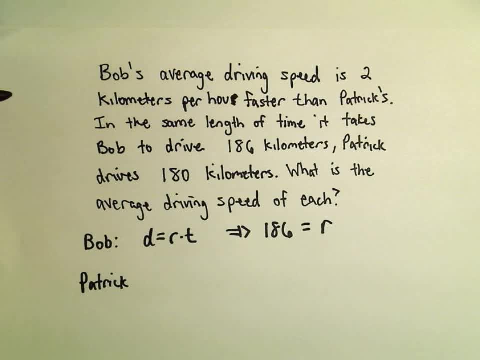 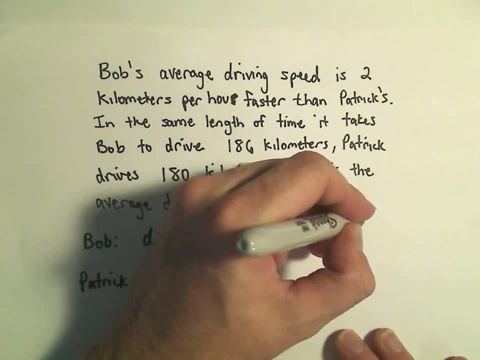 subscript here. Well, let's just leave it alone. We'll say that Bob's speed is r kilometers per hour, And we don't know the time either. We just know that it takes the same amount of time. Okay, so for Patrick, it takes in 186 kilometers per hour. 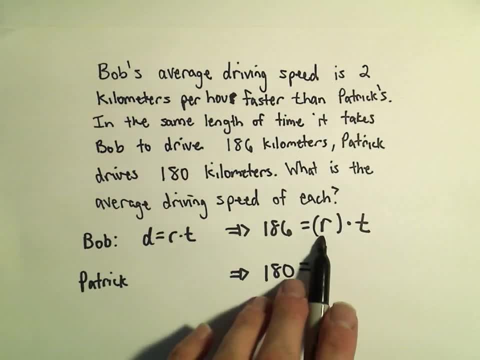 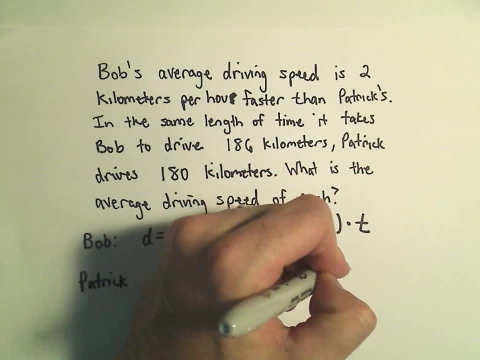 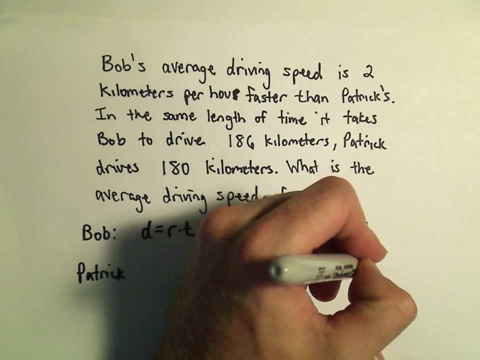 So that's 180 kilometers. Okay, if Bob's rate is r, we know that he's going two kilometers per hour faster, So my rate would have to be, well, his rate minus two, because I'm going two miles per hour slower. But again, we know that it's the same length of time. 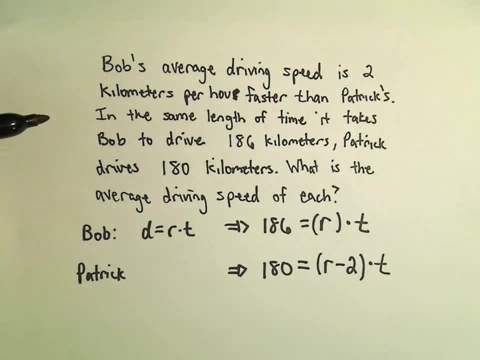 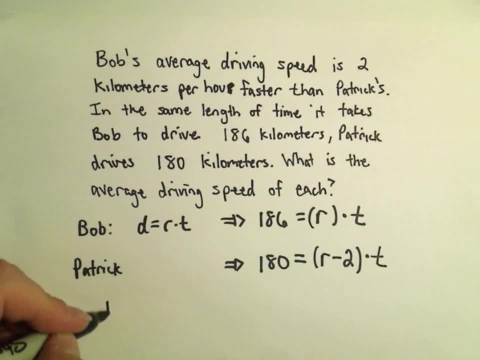 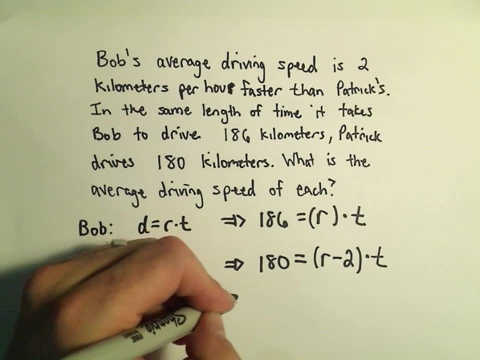 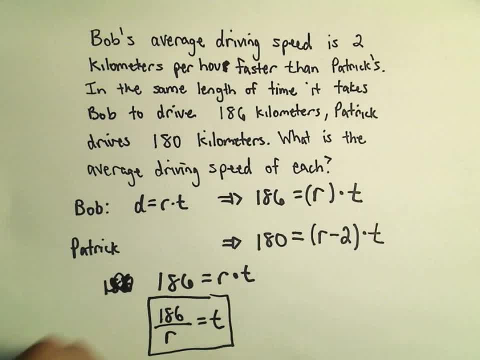 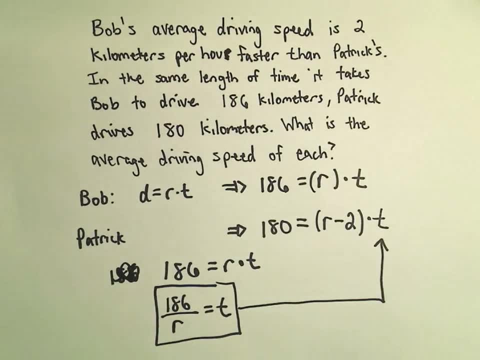 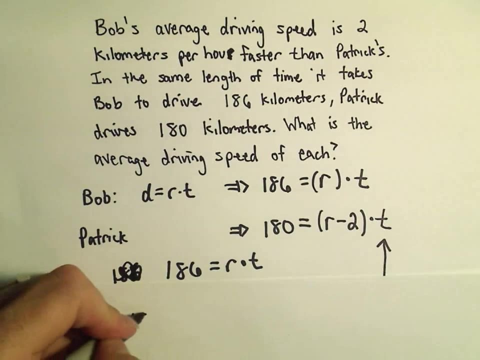 t. And again, what I'm going to do is I'm going to plug that into the other equation for t and then I'm going to solve. All right, sorry, I was finding some more paper here, So we've got 180 equals r minus. 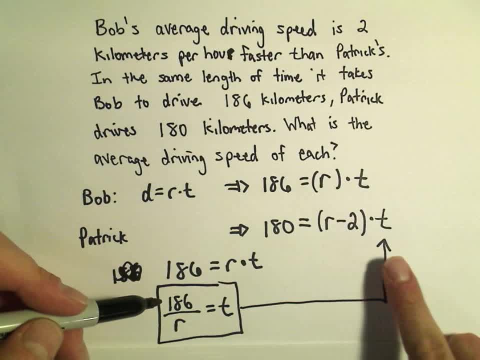 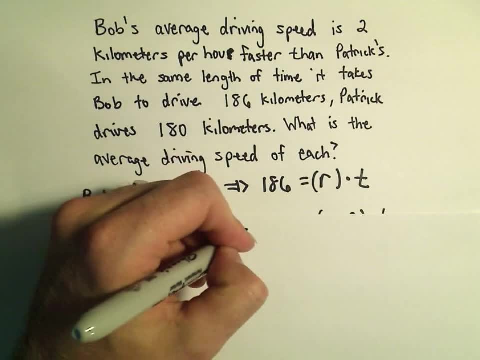 two. But again we solved the other one for t, so I'm going to plug it in for this t. But we said t is 186 divided by r. so I'm going to plug that in 186 over r And notice. 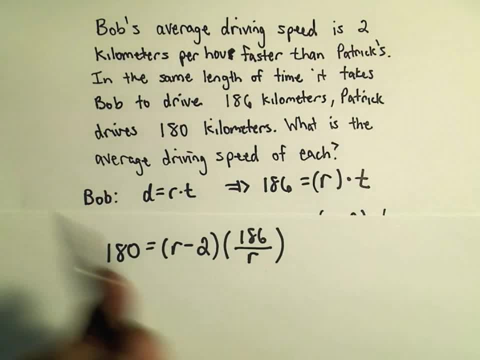 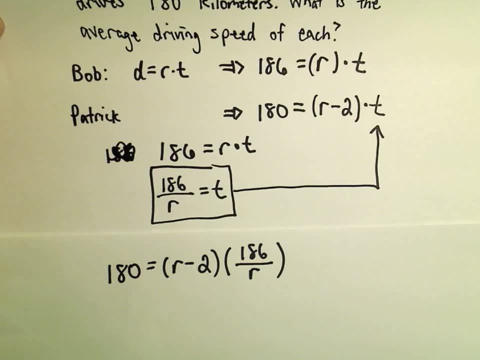 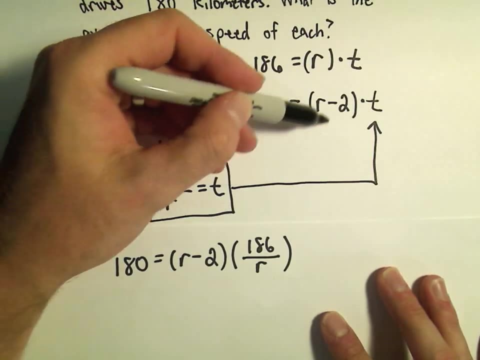 now I've got an equation involving just a single variable, only r, And that's always a good thing, because then you can usually Solve them and find the value without- at least in this case, hopefully without- too much trouble. All right, so again, just solve the first one for t. plug that into the second one. 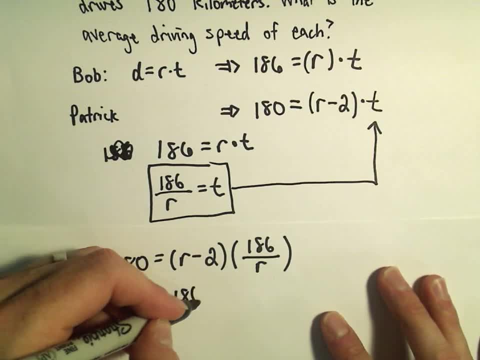 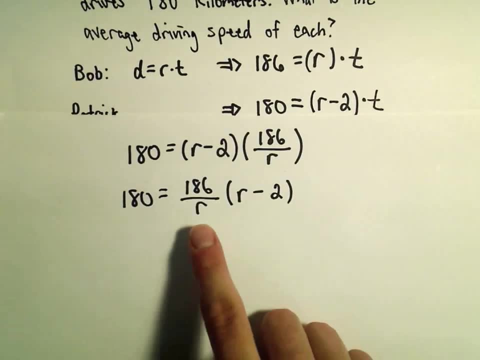 So what I'm going to do is I'm first going to rewrite. I'm going to rewrite 186 over r out front, Then we have r minus two. What we're going to have to do is we're going to have to distribute this 186 over r to both sides- Or, excuse me, not to both sides, but 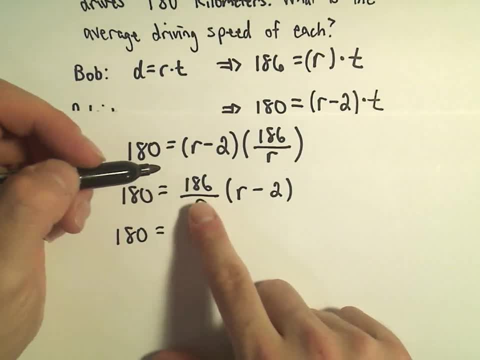 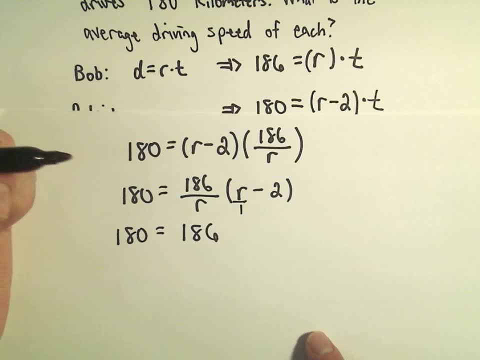 to both terms and sides. If I take 186 over r and multiply by r, the r's would simply cancel out, So I would be left with 186.. And then if I distribute the 186 divided by r to the negative two, I would 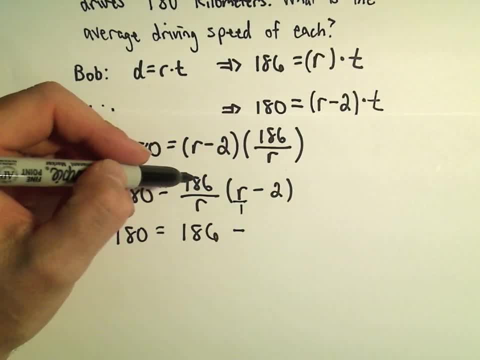 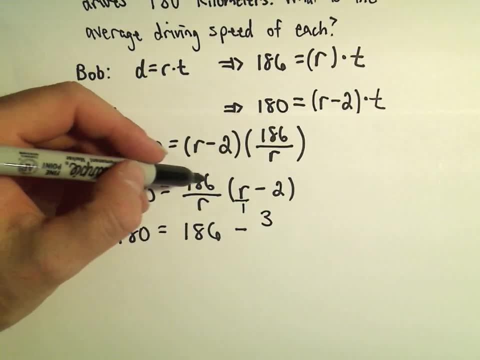 get negative. Okay, so if we take two times 186, let's see what is that That would be, I believe Let's see. so two times 200 would be 400.. That's 14 away. so we should take 28 away. 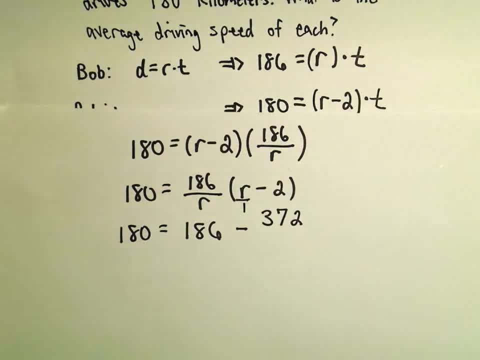 from 400.. So how about 372?? That looks pretty good to me. Double 180's, 360, and another 12.. Okay, over r, and you could have done okay. so what I'm going to do now. Um, notice we. 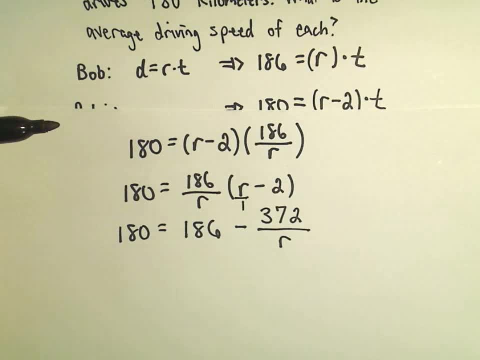 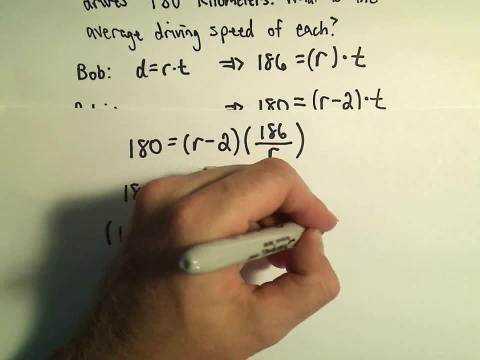 still have this r floating around. What I'm going to do in this case is to get rid of the r. I'm going to multiply both sides of this equation by r, So on the left side, we'll have 180 r. On the right side again, I'm going to fortunate, So I'm going to. 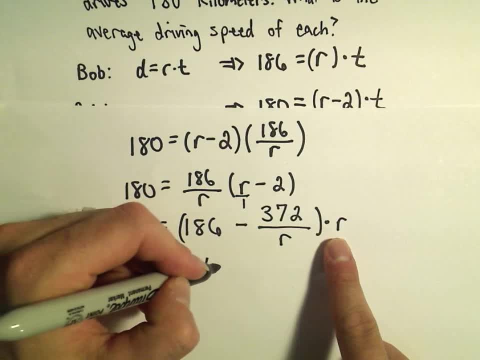 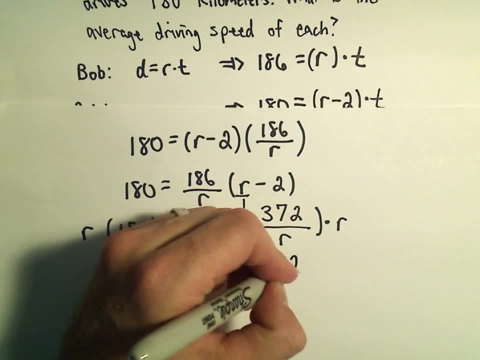 Again, I have to distribute. so I would get 186r When I multiply it to the negative 372 over r, those will cancel out. So a little bit of algebra here And now we're getting pretty close, Okay, so I'm going to subtract.